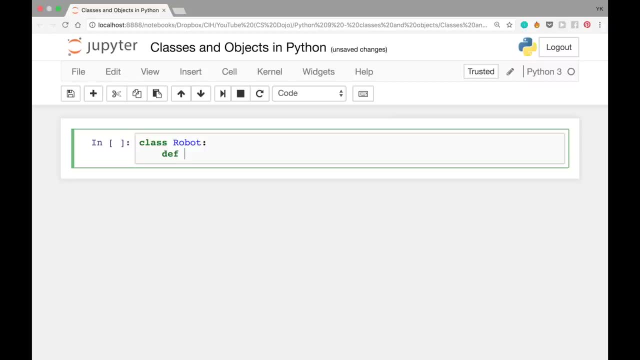 Introduce self. For that you can just write def, introduce underscore self, parentheses, colon and four more spaces after that, And then print Double quote. My name is plus self. that name And this keyword here, self, is sort of like this in Java and it will refer to whatever object we're running this function on. 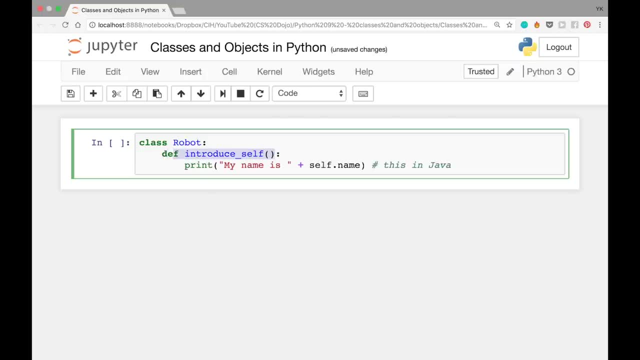 So, for example, if we run this function, introduce self on an object whose name is Tom, this is going to print out: my name is Tom, because self will refer to that object. Now, this function, you know, if you see. 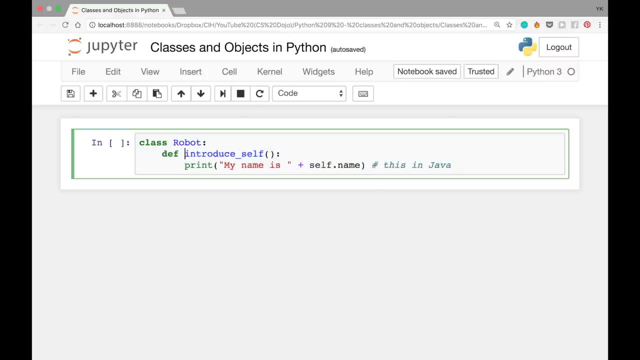 It looks like a regular Python function. We're defining a function called introduce self and then below that we have some implementation. But actually, when this function is within a class, when this function is a method of a class, you need to add an additional argument and that's going to be called self. 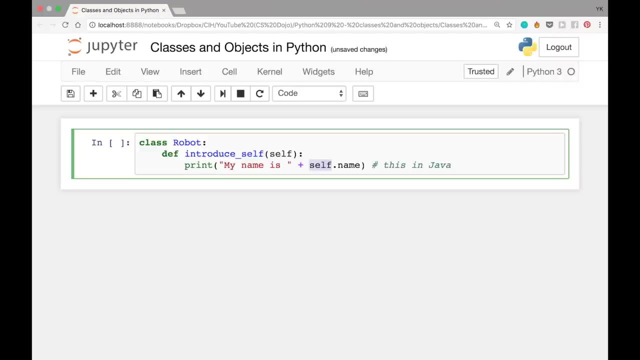 So this self is exactly the same as this self right here. So in Python, basically, you need to add this additional argument called self to every method you want to add to this class And once you run this block of code, this class is going to be created and you might say: what about the attributes, like the name, weight and color? 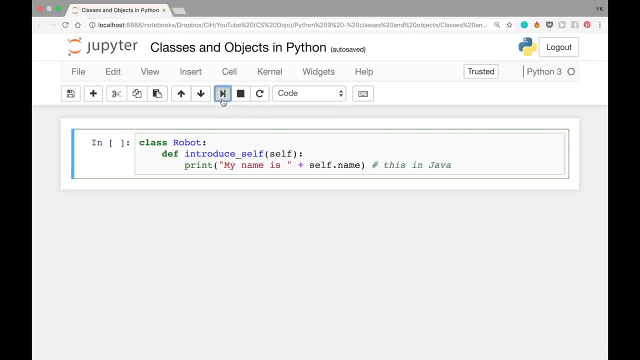 We're going to worry about that later, So let's run this block of code for now. Now that we have defined this class, we'll be able to create an object out of this class. To do that, you can just write: R1 equals robot parentheses. 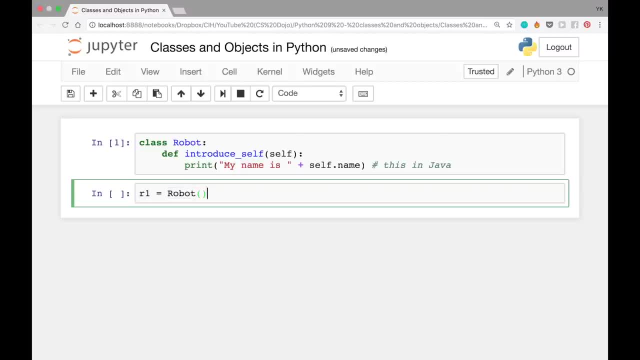 Again, note that the word robot is capitalized here and this simply says create, Create- Create a new object with the class robot, And here you're using the default Python constructor for this class robot, And to set the attributes you can just write: R1.name equals Tom, R1.color equals red and R1.weight equals 30. 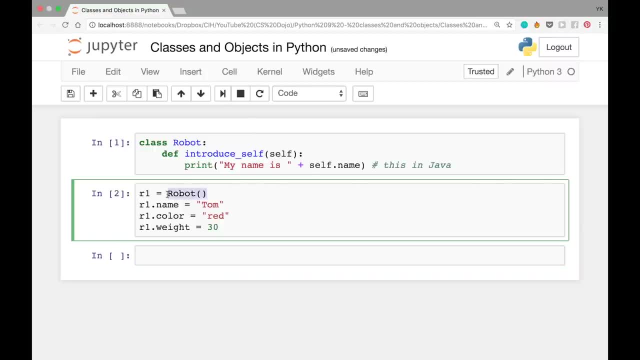 And when you run this cell, a new object has been created, It's assigned to R1 and then its attributes have been set And then, if you want to run this function, introduce self on this object, you can just write R1.introduce self- parentheses. 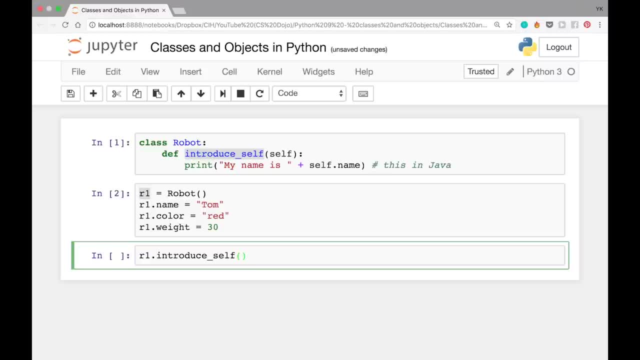 And you don't need to pass in any arguments here. And when you run this cell, what's going to happen is it's going to go into this part of the code and then self will refer to R1.. And so this part of the code will look like print. 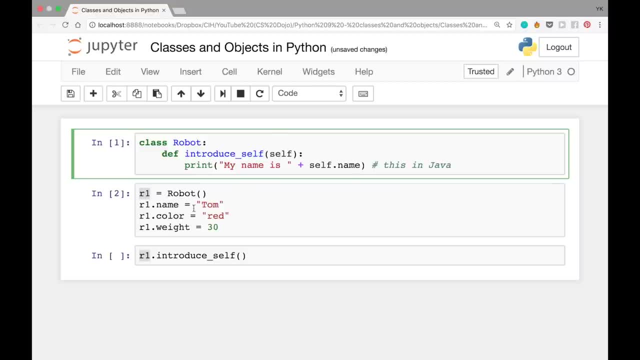 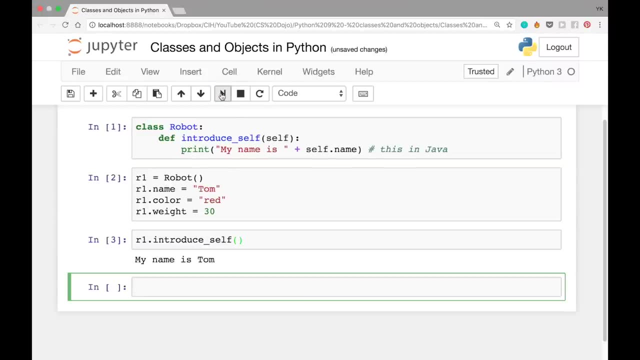 My name is R1.name and R1.name is of course Tom here, So it should print: my name is Tom. Let's see if it works. And it did. We see, my name is Tom right here. And just like that, you can create another object too. 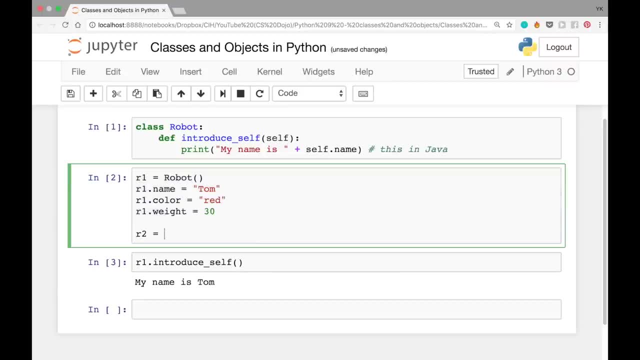 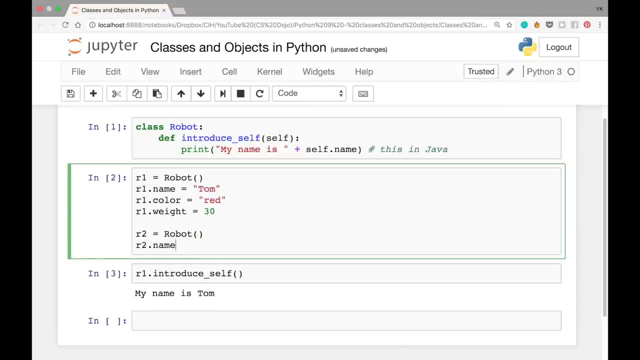 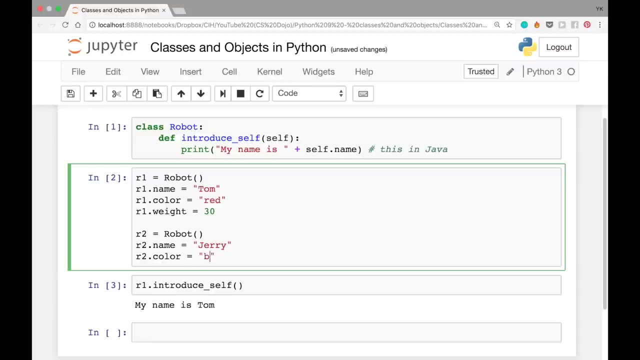 Let's go back into this cell and let's write: R2 equals robot. This will create a new robot object, And then let's set its attributes too, So R2.name equals Jerry, R2.color equals blue And R2.weight. 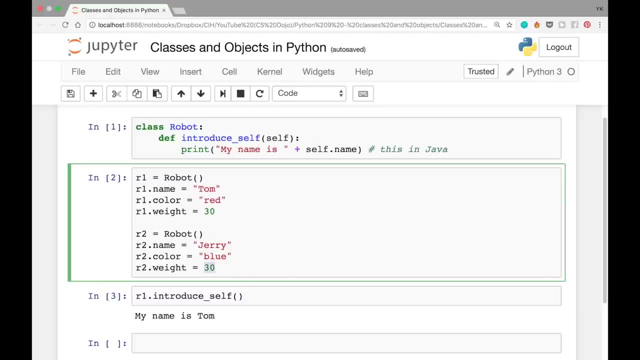 equals 30.. Let's actually set the weight of R2 to 40, like we saw earlier, And once you run this cell, you'll have an object in R1 and another object in R2, with different sets of attributes, of course. 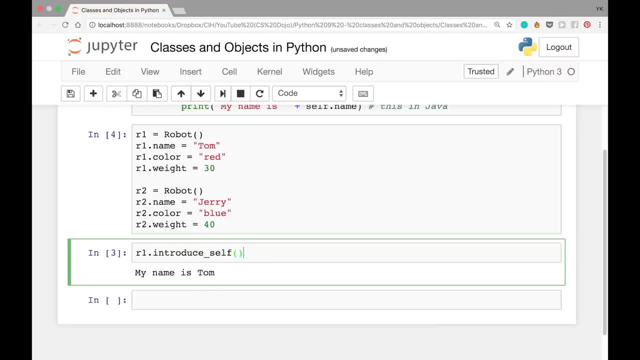 And then at this point you should be able to run R1.introduce self and R2.introduce self. So the first line should print my name is Tom, just like we saw earlier, And then the second line should print my name is. 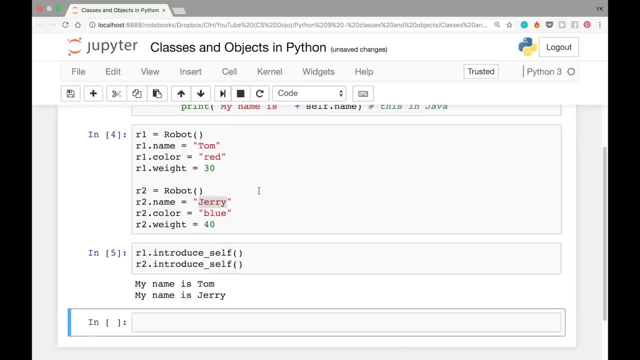 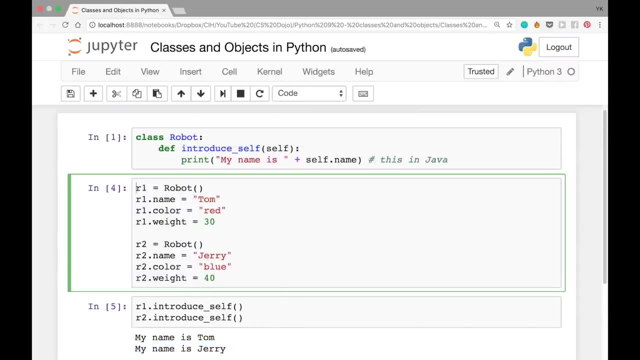 Jerry instead. So let's see if we can get that. And that's exactly what we see. Okay, Going back a little bit, when you see this block of code that we use to create these two objects, you might say, well, that's not great, because here we're writing: R1.name equals Tom. 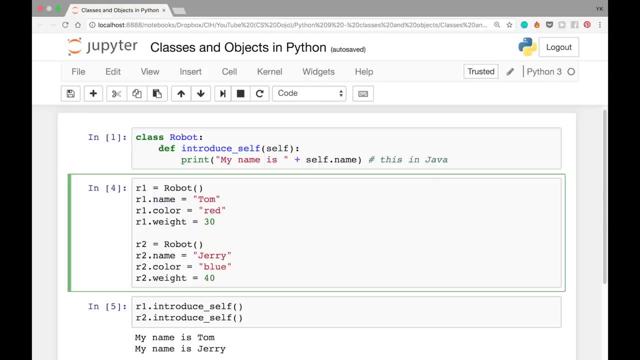 But if we misspelled the word name, for example, if we wrote R1.name equals Tom, it's going to stop working. Okay, Because if you look at this function in particular, in this class we're writing here: print: my name is selfname. 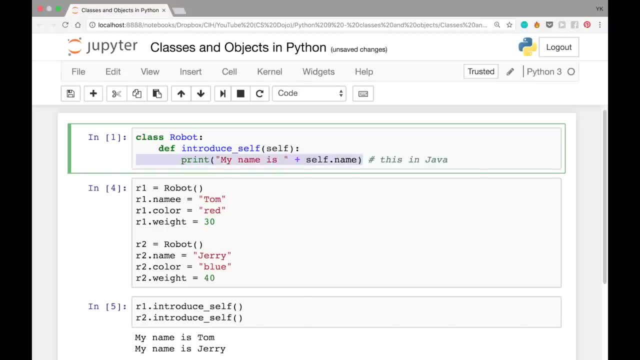 And this piece of code basically depends on us writing the attributes name name correctly for it to work. What I mean by that is, for example, you know, if you misspelled the word name by writing R1.name equals Tom. the attribute called name does not exist in this object anymore. 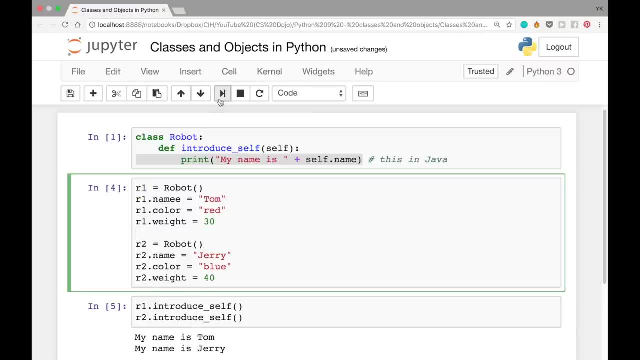 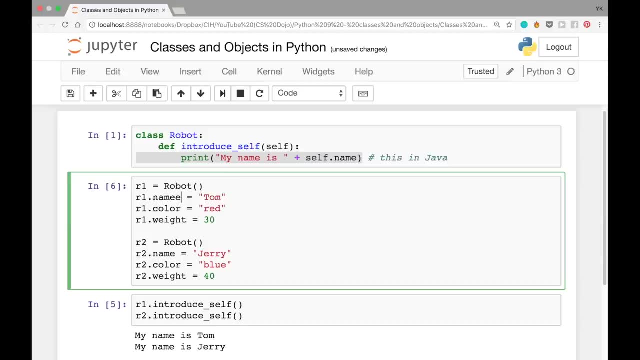 So we can actually see what's going to happen if we try that. So let's run this cell again. And this is not going to give us any error, because when you write R1.name equals Tom, the attribute called name is just defined. 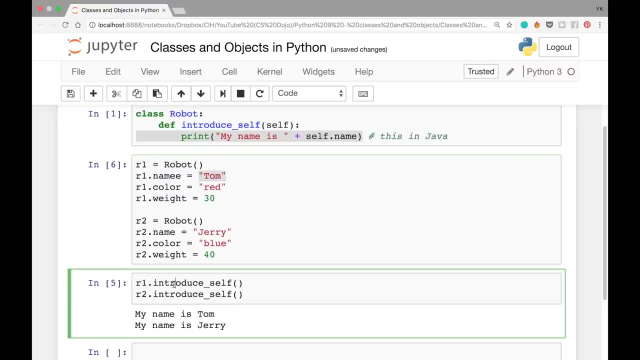 And then the value Tom is set for that. But when you run this block of code R1.introduce self- let's comment out the second line and let's focus on the first line. When you run this part you'll say attribute error. 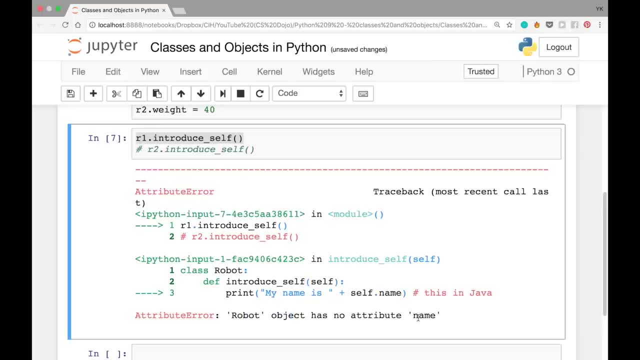 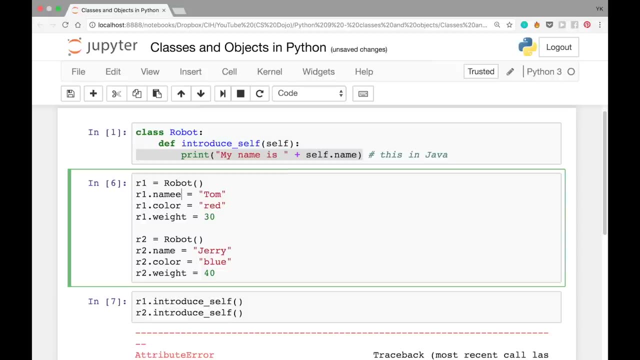 And it says Robot as object has no attribute name and that's because it has the attribute name- me- but it doesn't have the attribute name. So this is probably not the best way to deal with different attributes we have. Let's see how we might be able to fix that. 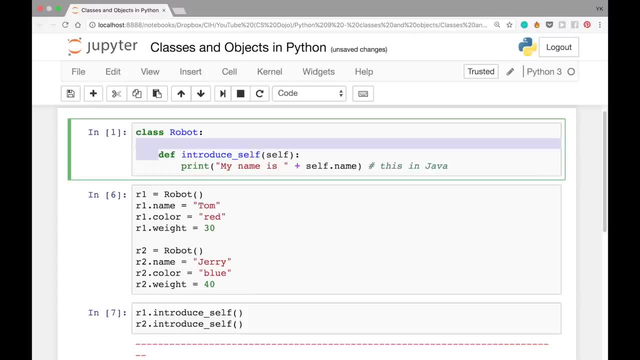 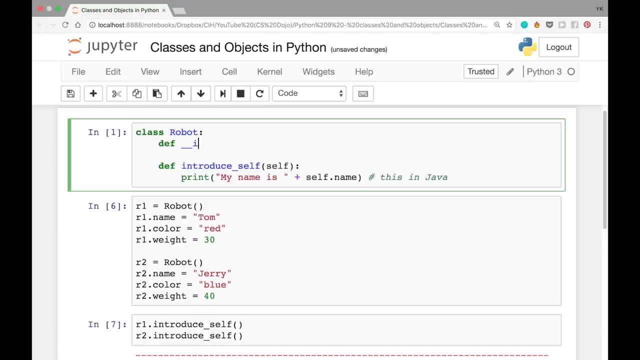 And the way you can fix it is basically by using a constructor, And in Python you can create a custom constructor with this keyword: underscore, underscore, init, underscore, underscore. So there's the word init, And it's surrounded by pairs, two pairs of underscores and then parentheses. 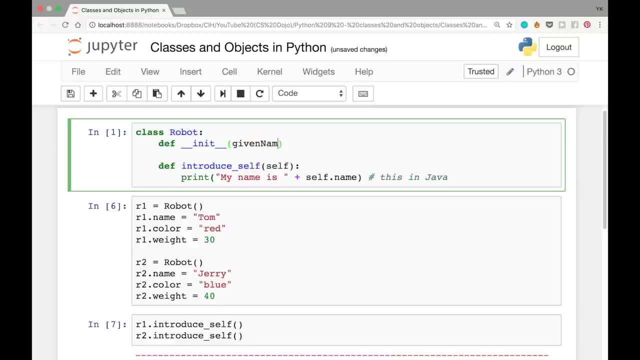 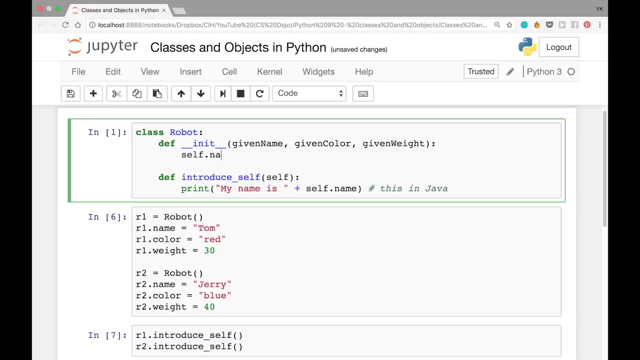 And let's have this function. take three arguments: given name, given color and given weight. So these are the name, color and the weight we want to set for this particular object that we are trying to create, And then we can write here: selfname equals given name, selfcolor equals given color. 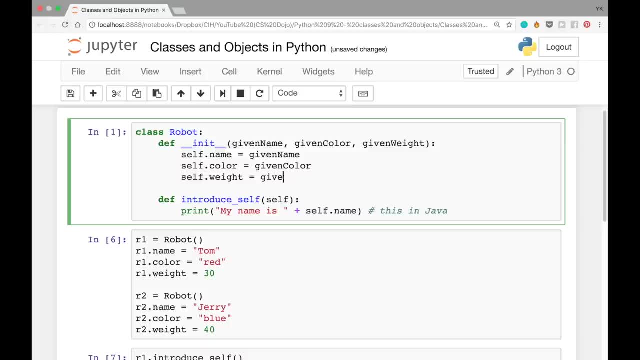 And this block of code of course says: set this object that we are just creating, set the object's name to given name and set the object's color to given color and set the object's weight to given weight. And earlier I said you need to add this self keyword, this additional argument, to every function we define in this class. 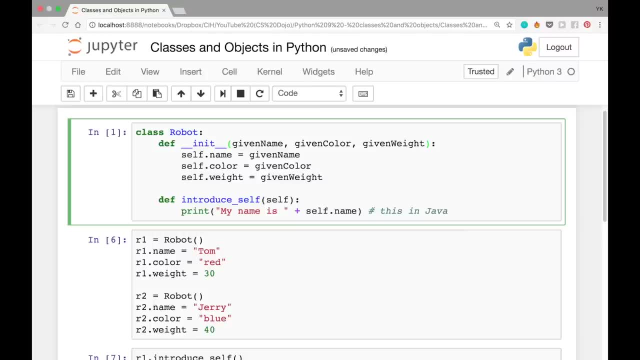 And the constructor is no exception. So you actually need to write self as the first argument, and then the arguments that you want to add in, And actually, just like many other languages, a common practice here is to name these arguments exactly the same as the attributes that we want to set. 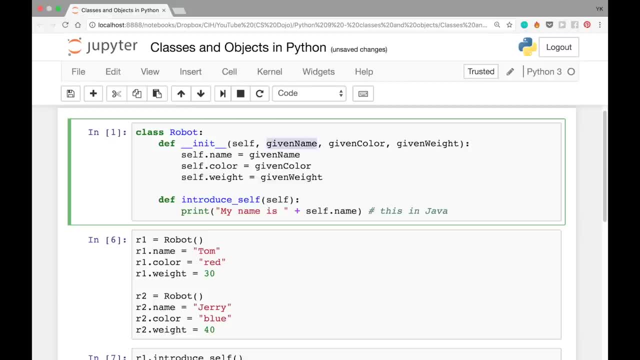 You don't have to do it, but that's just a style thing. So let's just do that. Let's change given name to name and then given color To color and given weight to weight, And once you run this block of code, this class is going to be refreshed with a new constructor. 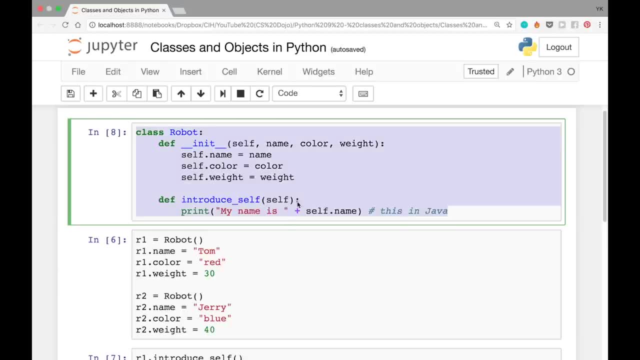 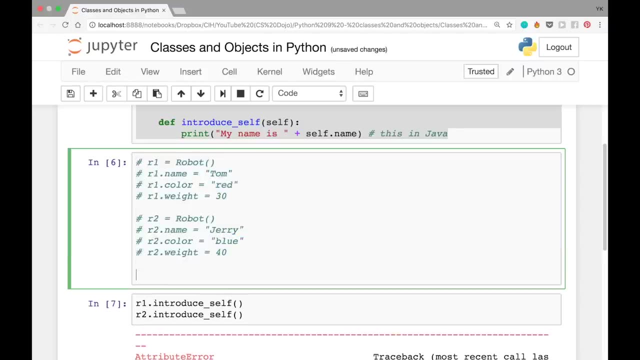 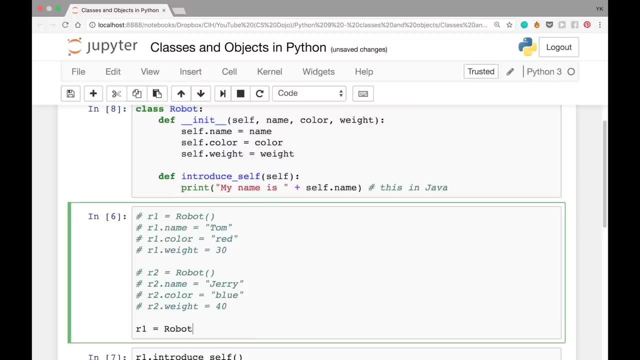 Once we have a custom constructor in our class, the default constructor that we used will stop working. So let's just comment out this block of code and then let's rewrite it using our new constructor. For that you can just write: r1 equals robot. 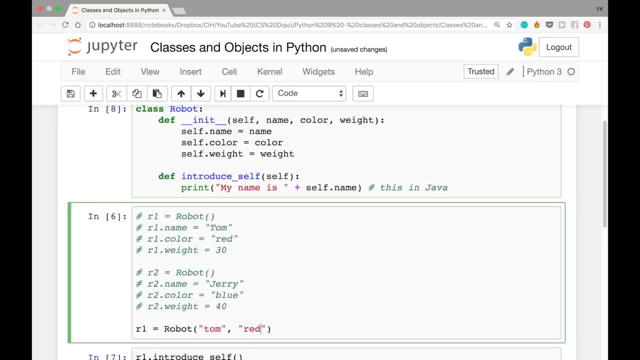 Parentheses: tom comma red, comma 30. Let's capitalize tom here, And then r2 equals robot jerry comma blue, comma 40. And these two pieces of code do exactly pretty much the same thing as what we saw earlier. 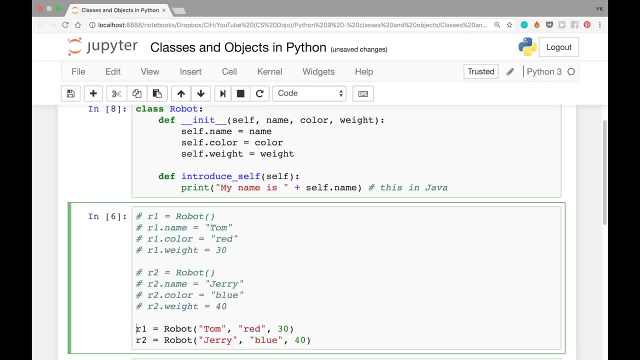 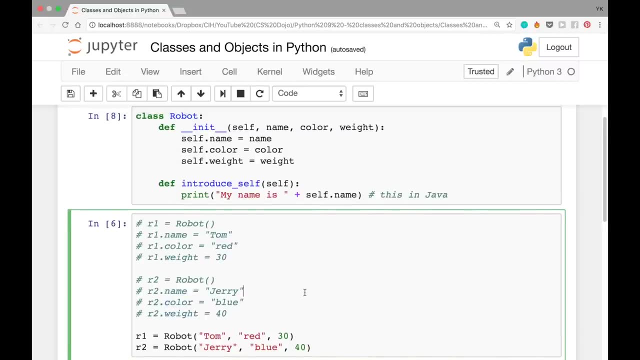 But, as you can see, this is much cleaner because you don't need to specify the attribute names manually every time. And just Just to reiterate, just to sort of clarify: this line r1 equals robot tom red 30, will create a new robot object. 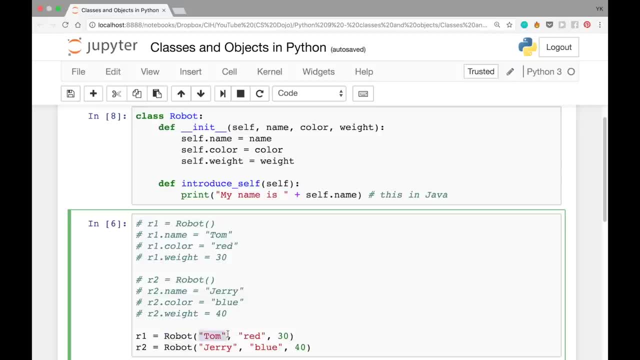 And then it'll set tom as its name, because tom will go in here as the name argument and then it'll go in here selfname, And self again will refer to the object that we're creating. So it's sort of like saying r1.name equals name, r1.color equals color. 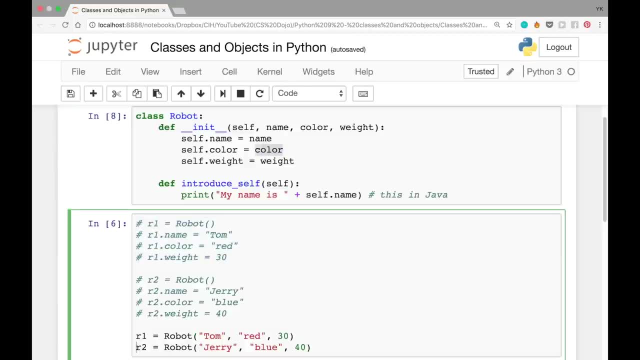 Just like we did, And of course, it's the same thing with r2.. Okay, and to make sure we don't have anything left from the previous code we were using, let's go to kernel and click restart and clear output. This is going to clear out every variable we defined earlier.